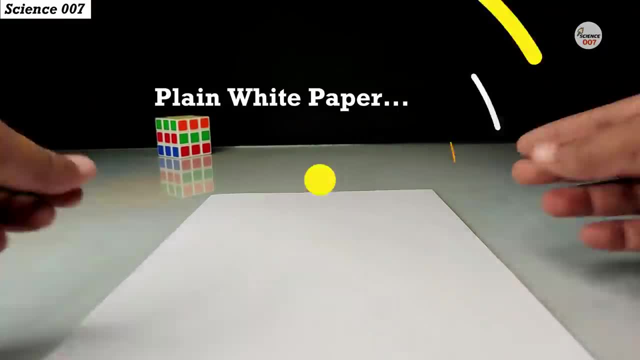 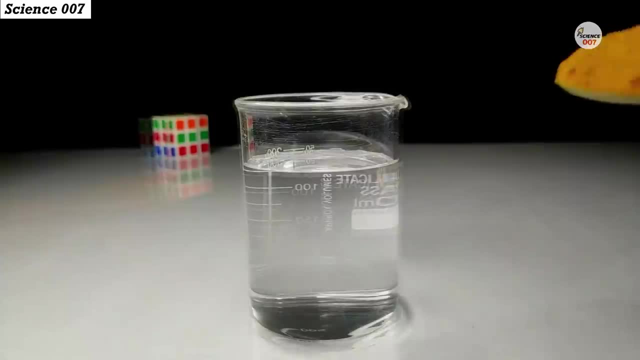 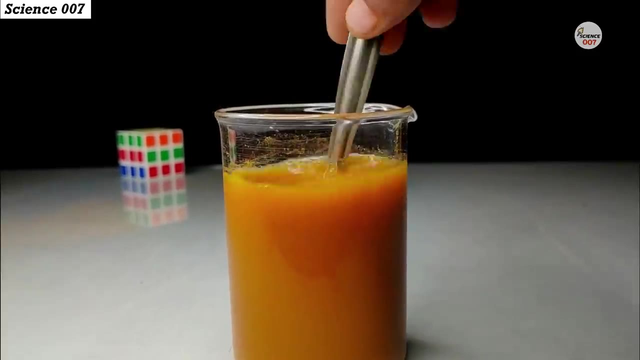 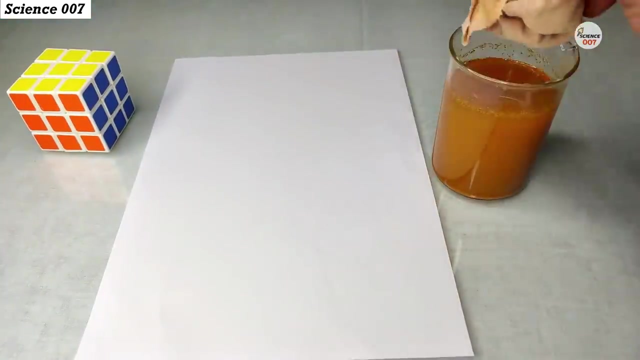 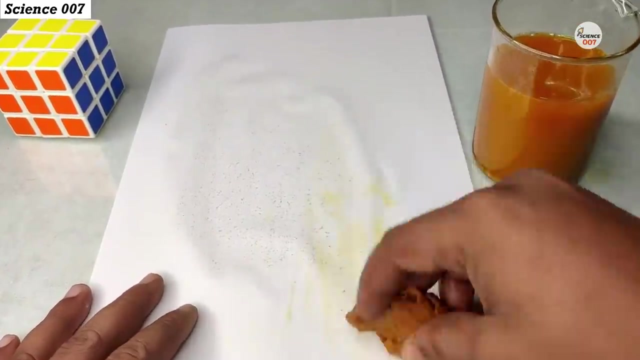 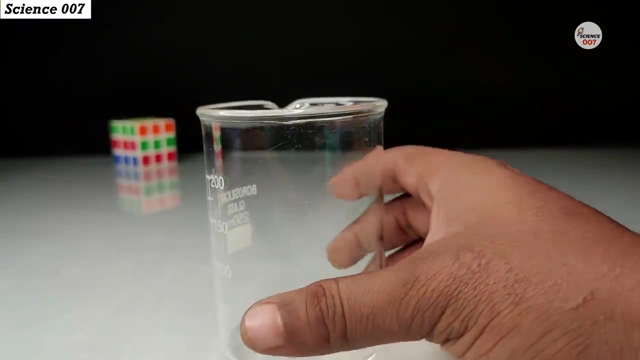 Please subscribe to the channel and press the bell icon to receive notifications when I upload a new video. Thank you very much for watching. Thank you very much for watching. Please subscribe to the channel and press the bell icon to receive notifications when I upload a new video. 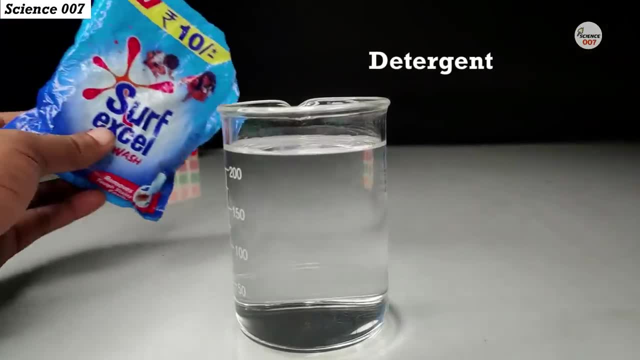 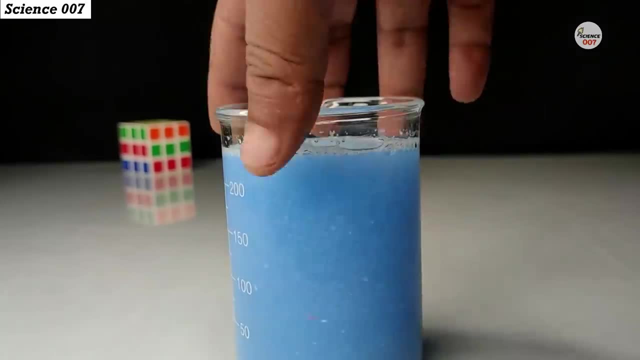 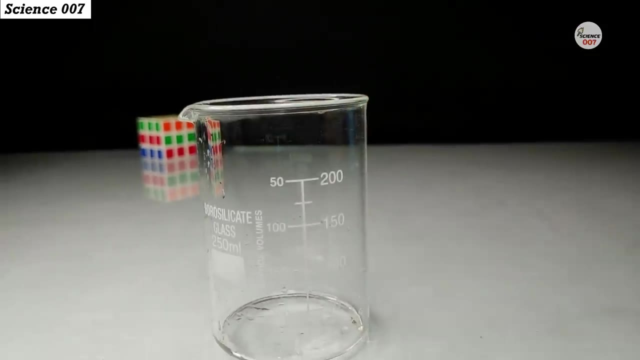 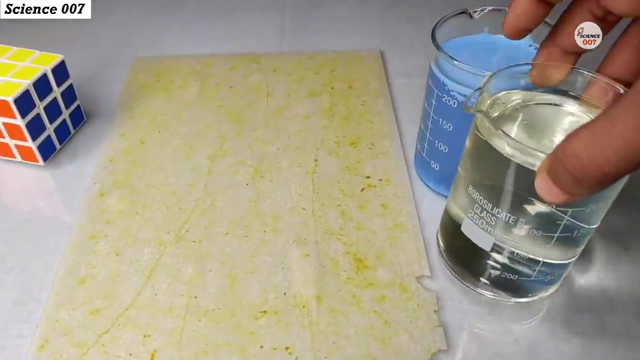 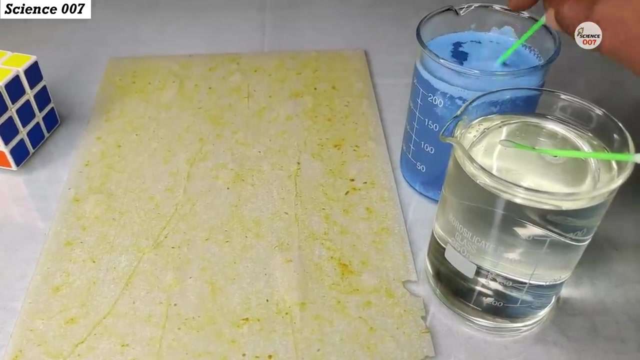 Thank you very much for watching. Thank you very much for watching. If you want to support us, please subscribe to the channel with an í Will puis. Thank you very much for watching. if you want to support us, please subscribe to the channel with an. i Will puis. 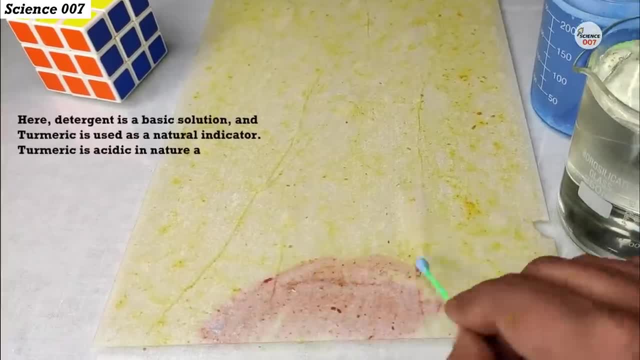 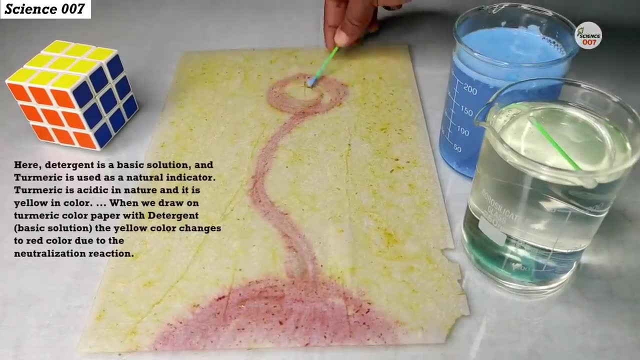 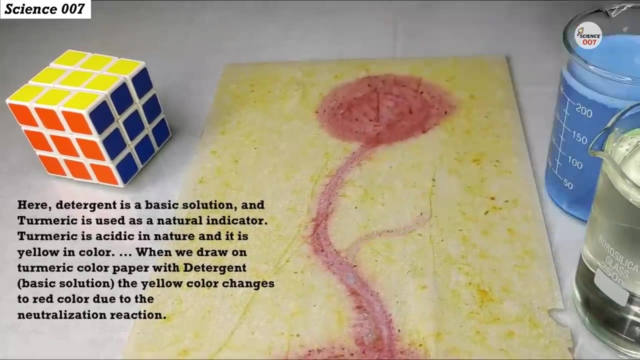 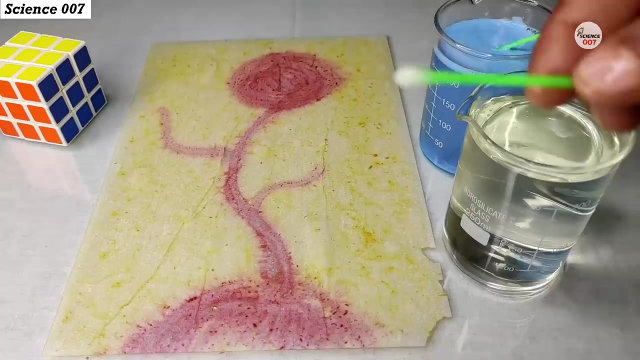 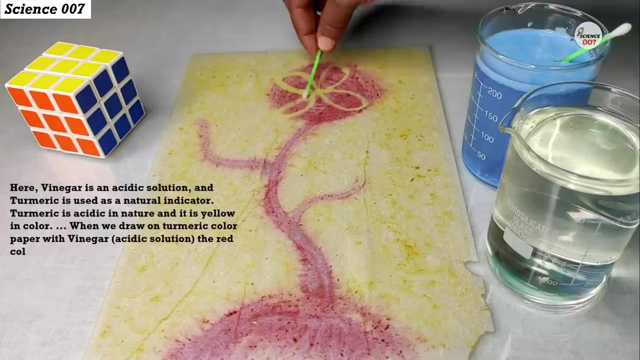 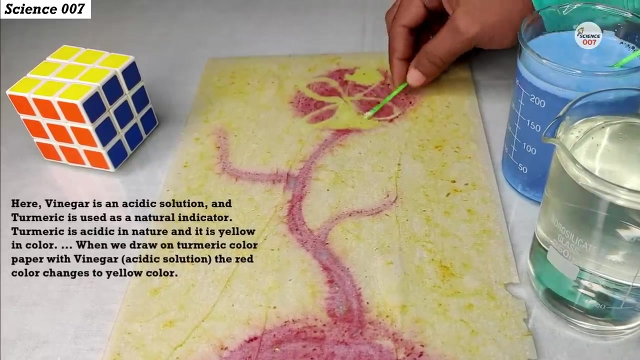 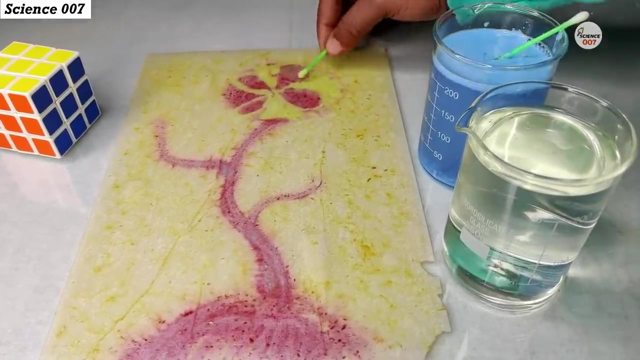 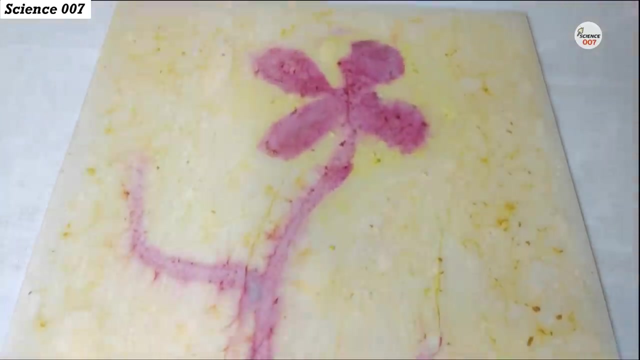 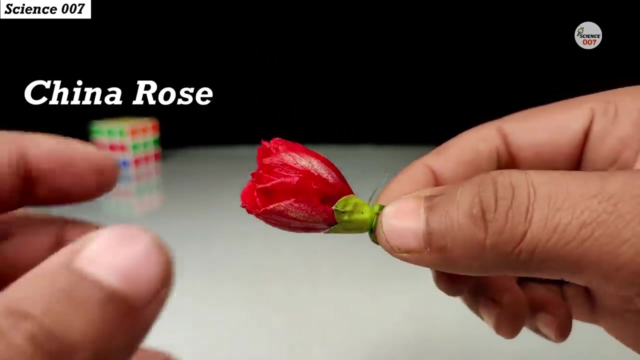 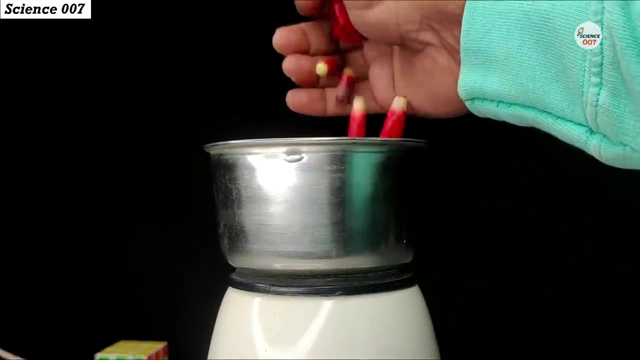 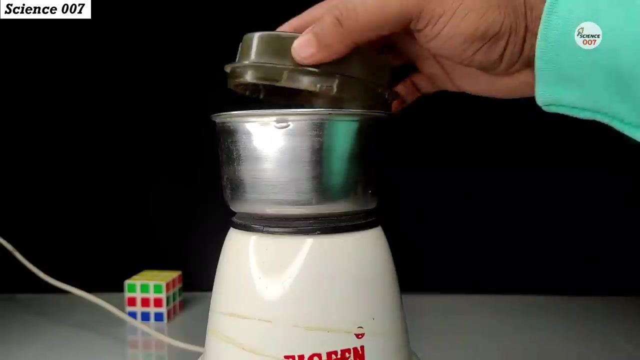 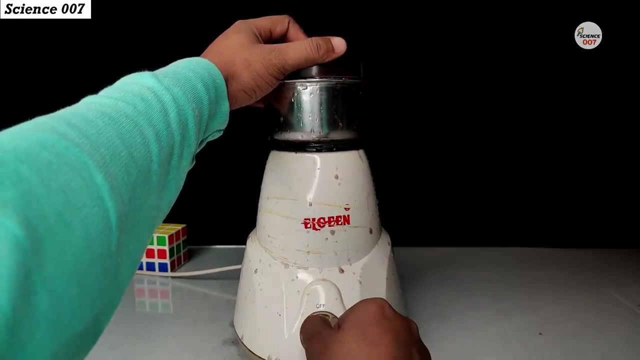 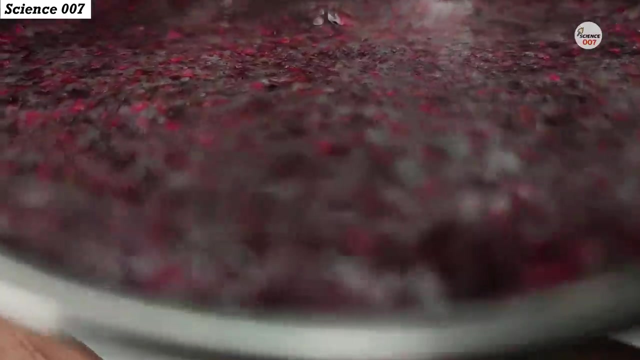 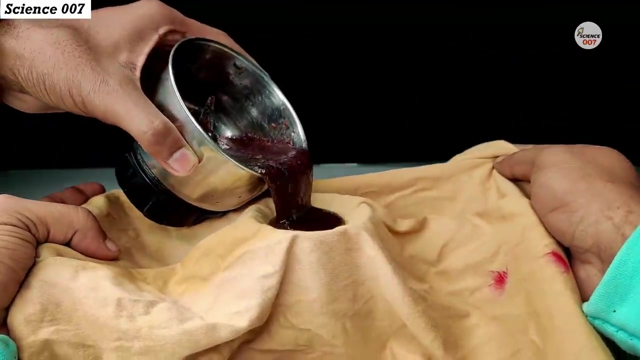 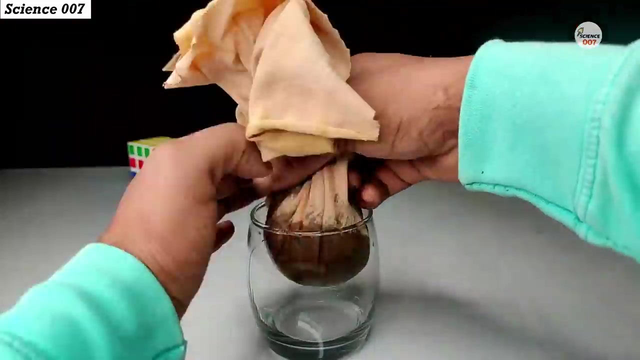 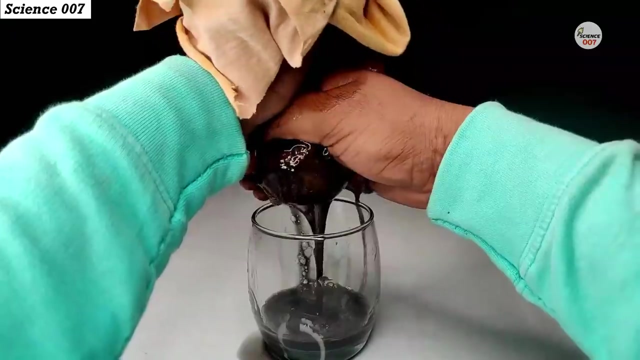 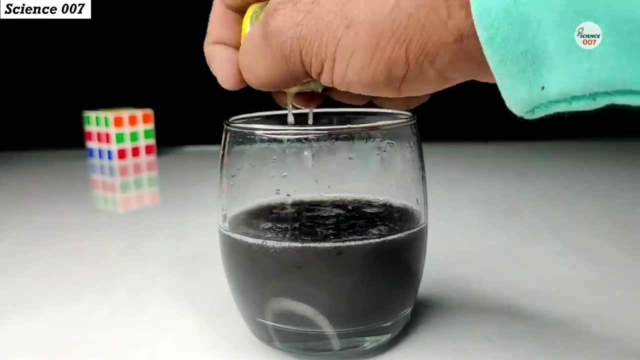 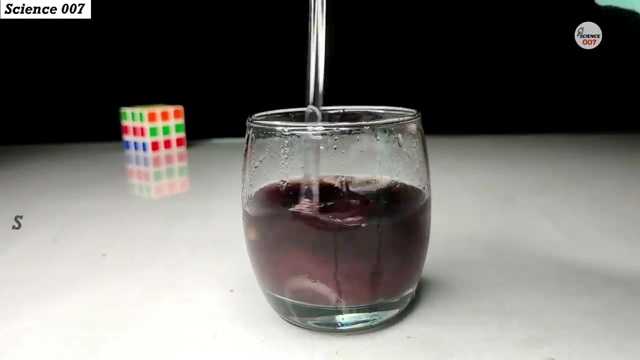 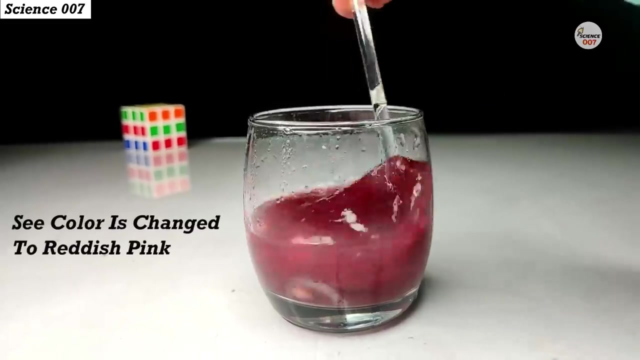 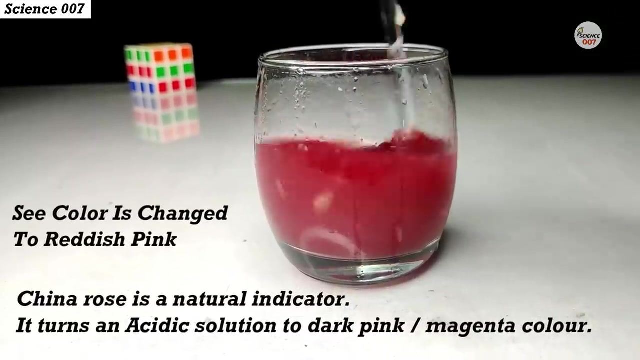 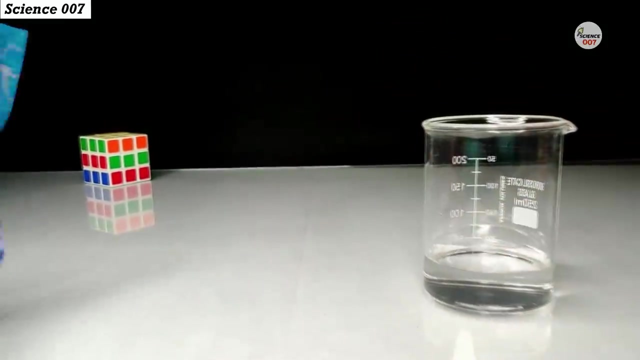 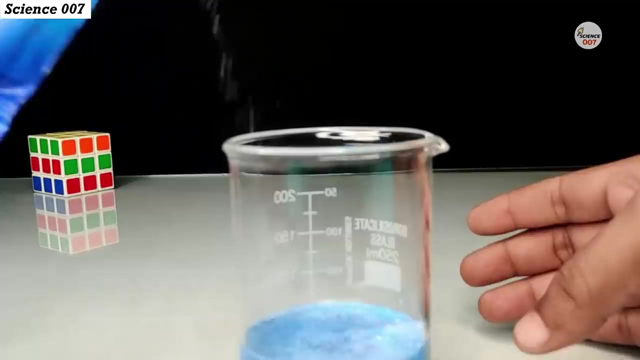 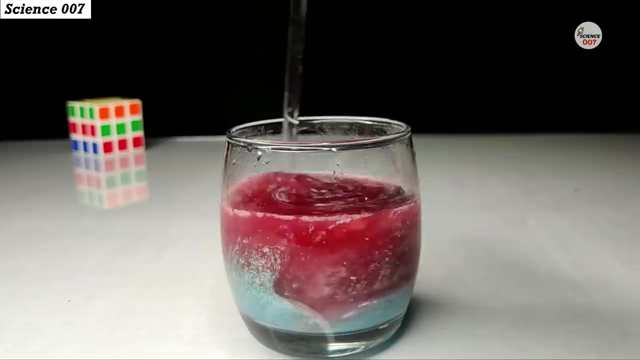 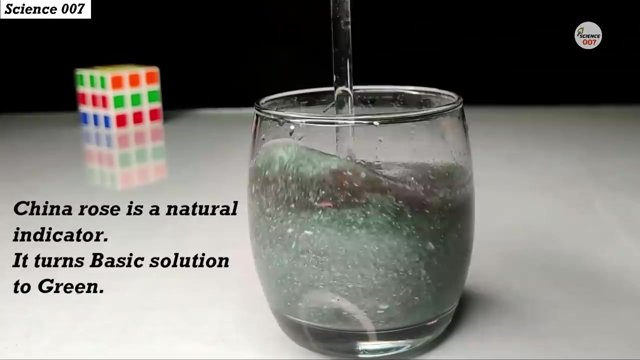 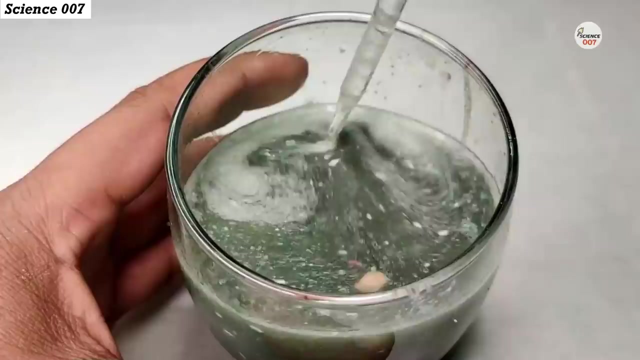 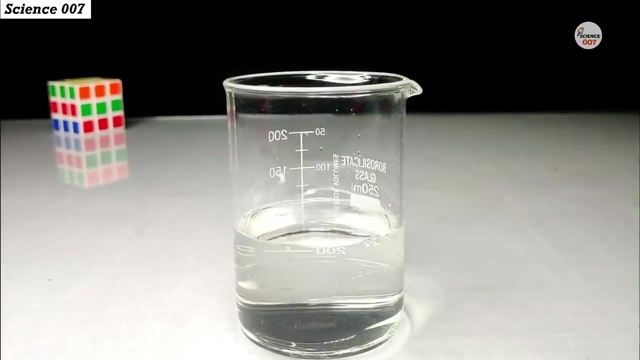 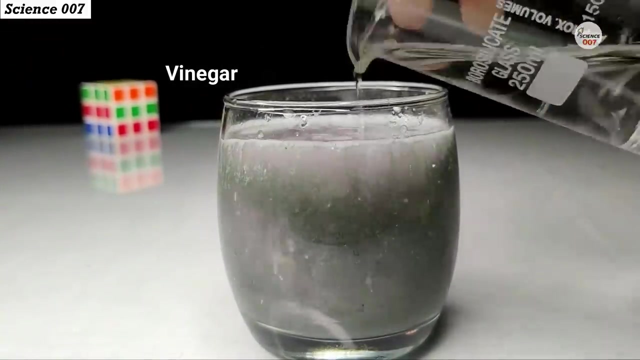 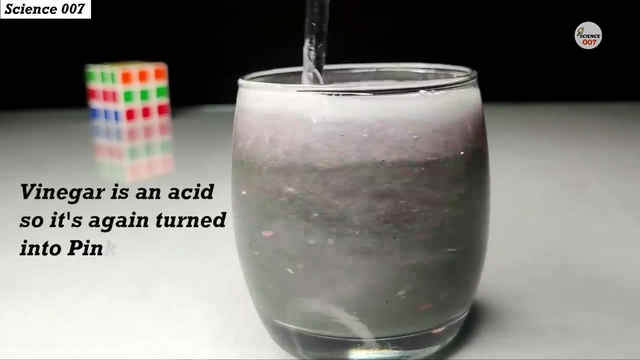 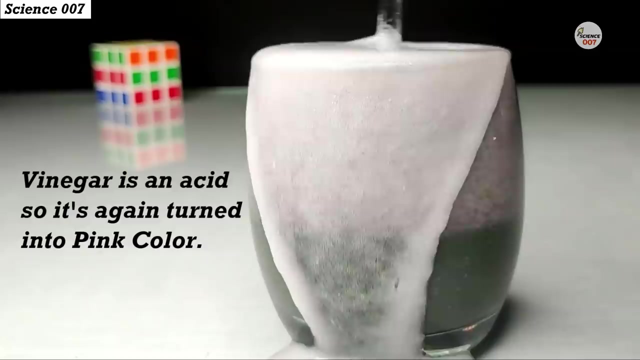 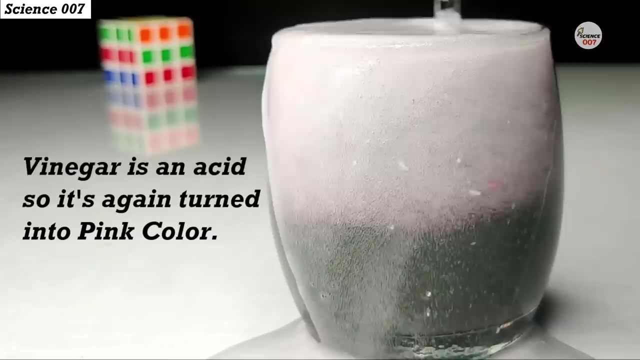